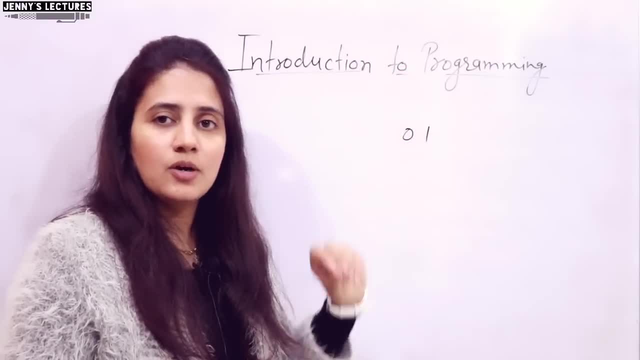 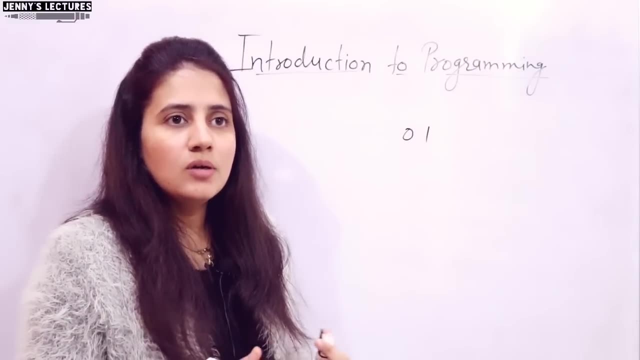 do that also. we'll discuss how that language, how that program will be converted into zero and one, and then computer will perform your task. fine, So basically you can say what computer run by programs. Computer is nothing without programs. It cannot do anything without programs. When you 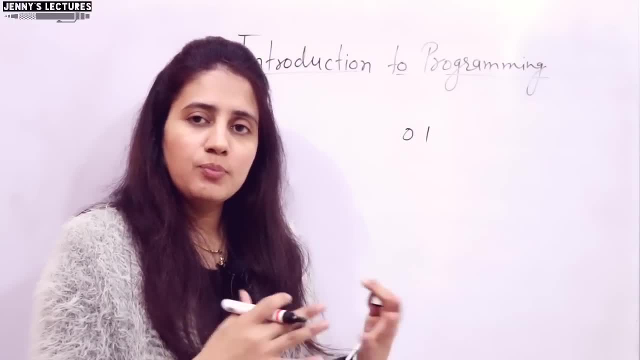 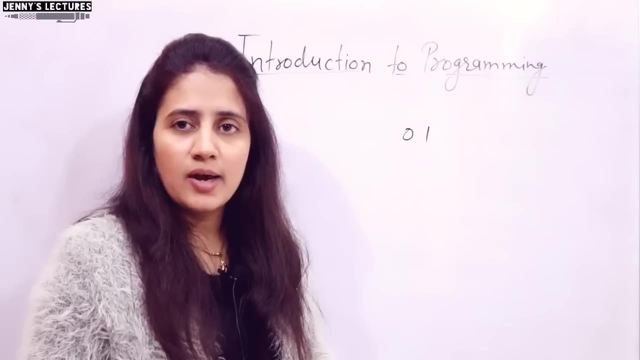 purchase a new laptop or computer that has already. you know many programs are already there in that programs, or you can, sorry, in your computer, Like some system programs, application programs, or you must have heard about system software, application software. Software is what Definitely. 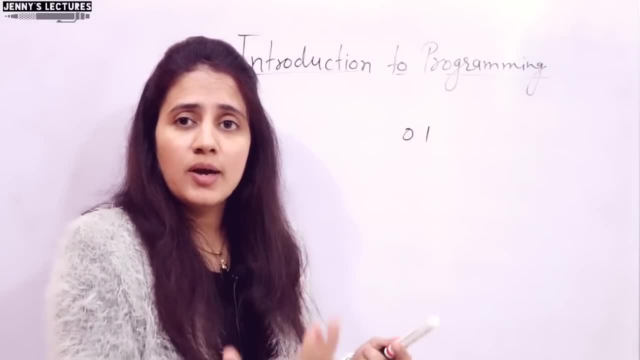 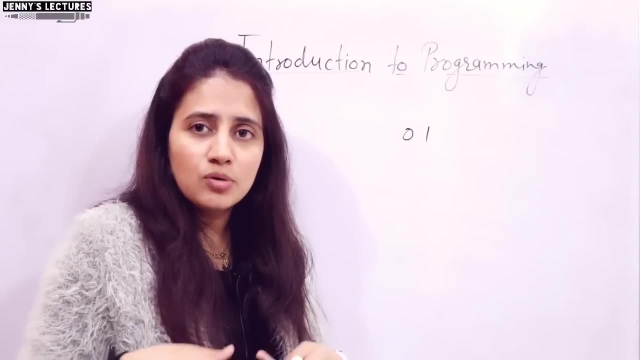 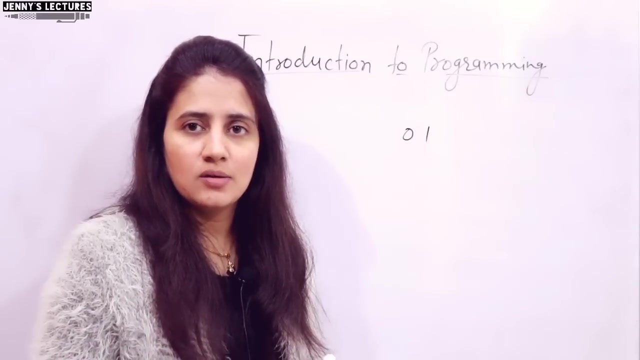 it is a set of programs, right? So system programs means what They are going to manage, that system resources. They are going to manage the hardware, and application programs or application softwares are what They are basically used to perform your task, your favorite task, Like web browser, is: 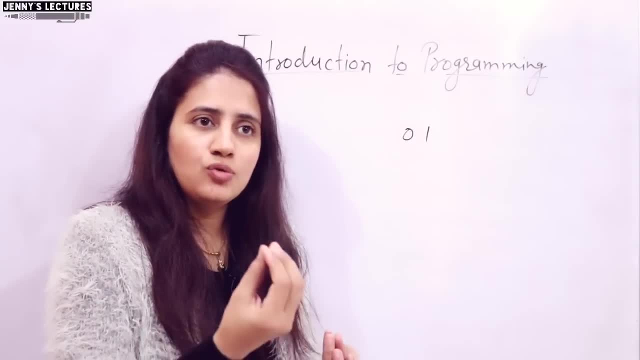 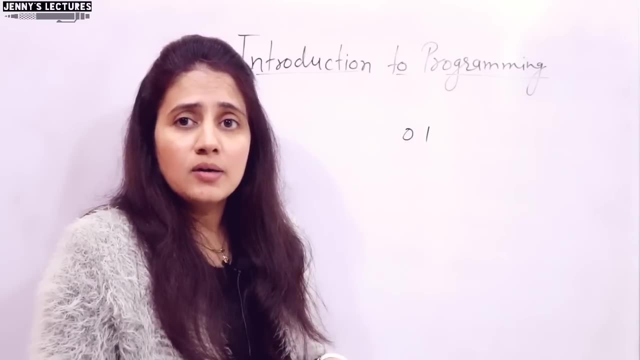 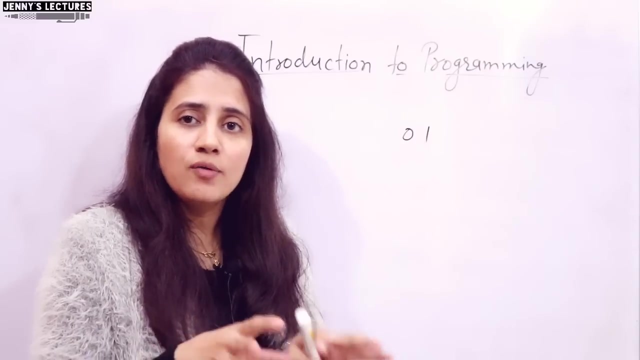 application software and text editor in which you you can edit, you can write text, you can edit text. MS Office, that is also a application software, right? But suppose, if you want computer to perform your task, any specific task, according to that you have to write, you have to write. 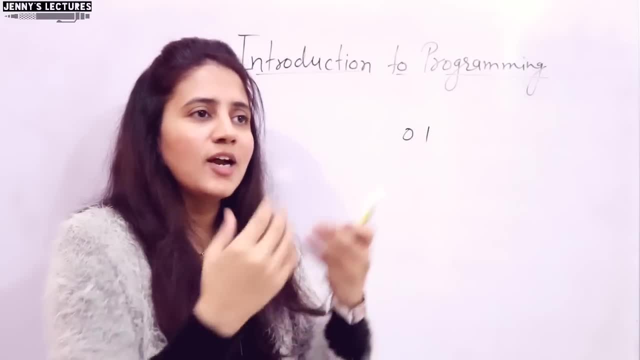 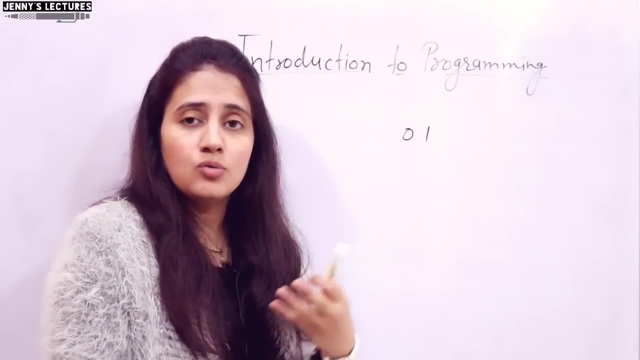 your own program and you have to submit that program. You have to give that program to computer and then computer will understand your program, or you can say those sequence of instructions and according to that will give you some output, right. So now, how do you write programs Like it's? 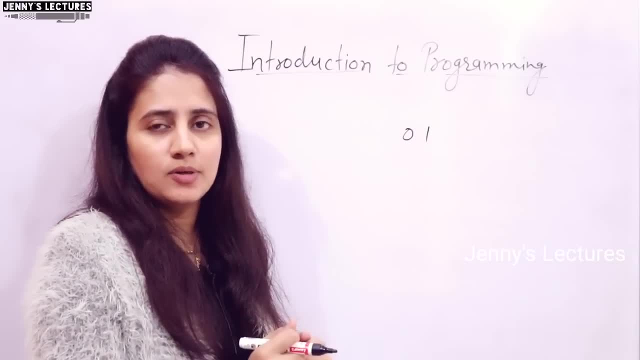 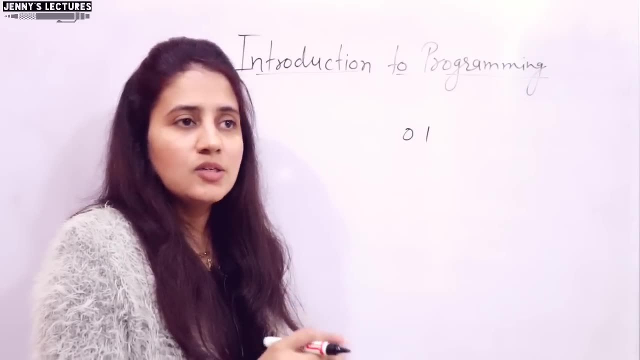 not like in simple English language, you will write programs and submit to computer. No, it is not going to understand. So for that thing we need programming languages, right? See when we communicate with each other, like if I want to write a program, I have to write a program. So 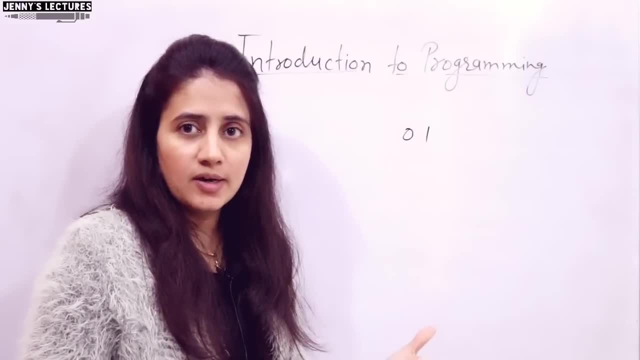 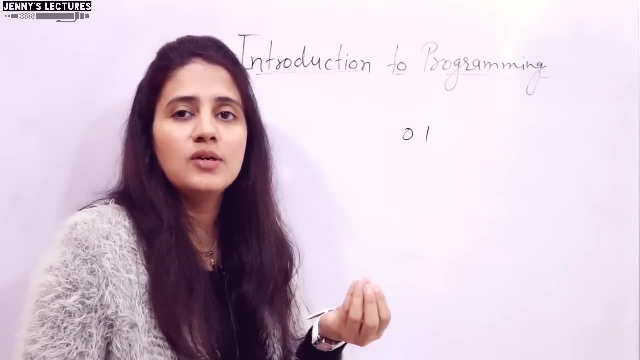 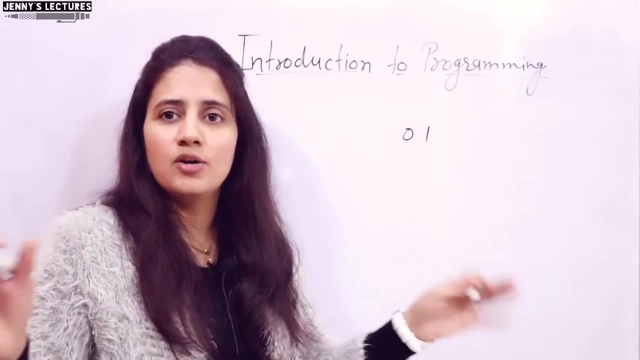 if I want to communicate with you, then the languages may be English, Hindi, right. So, and for communication, what? First of all, you need to understand the alphabets. First we study what: A, B, C, D, and then words. Then we frame sentences by using grammars and all right, And then we 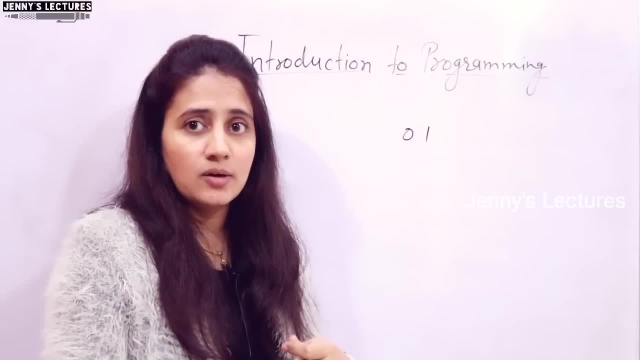 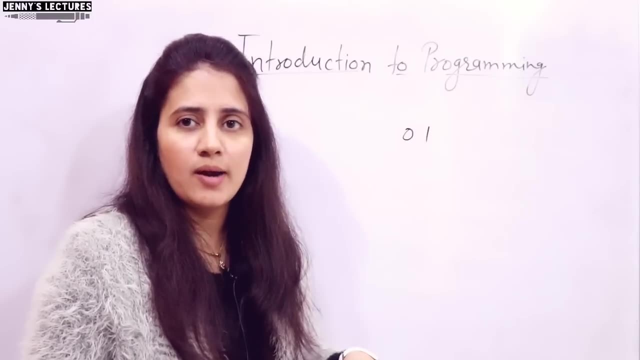 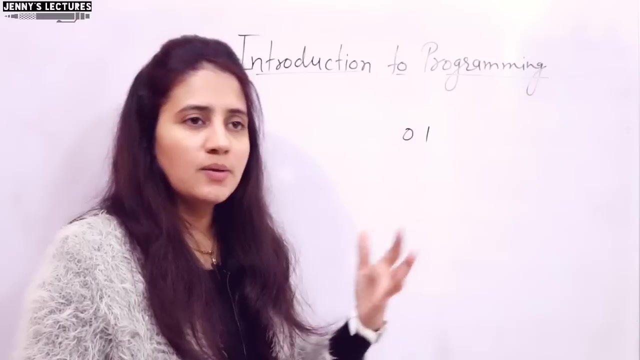 communicate, Then we frame sentences and then we communicate with each other. Same thing in language also. you need to learn something before writing the programs, Like the character set of that language, keywords and some syntaxes and some rules, right, And then 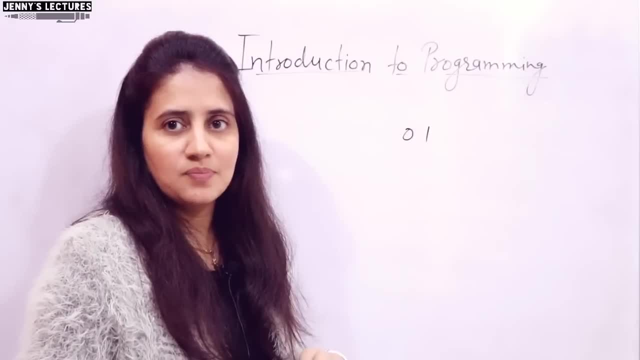 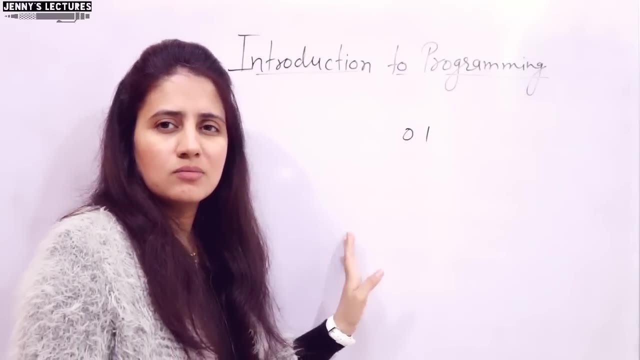 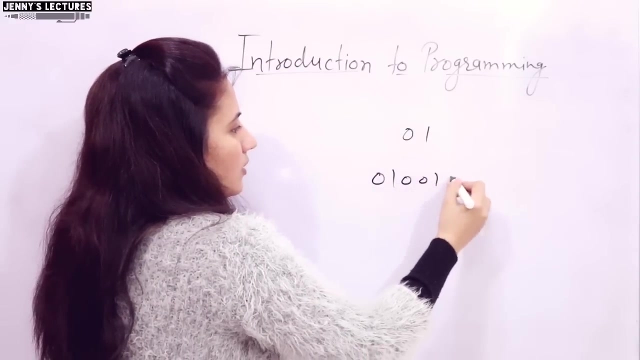 we can write programs and then we can interact with computers, right. But the point here is what computer can understand? only 0 and 1, and you are writing programs in what? If suppose C language, we take example of C language, then definitely we are not going to write like 0, 1, 0, 0, 1.. Suppose I. 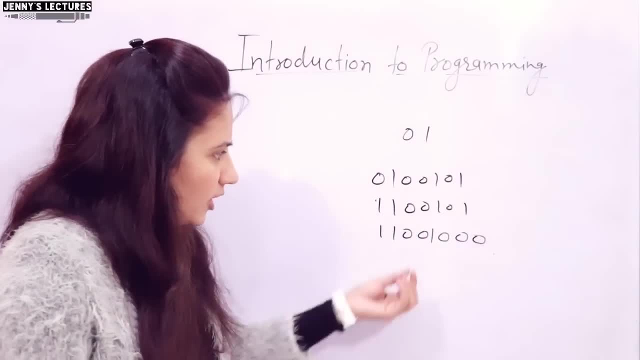 write this one. This is a bunch of 0s and 1s. So if I write 0s and 1s then definitely we are not. but we are not able to understand what is meaning of this thing. right, But maybe computer can. 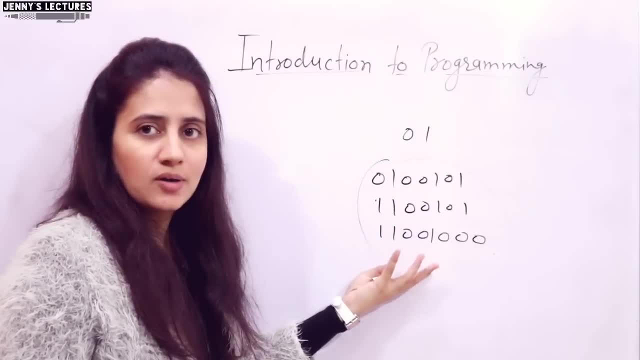 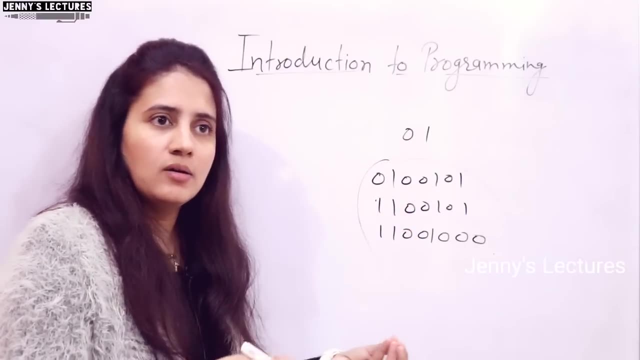 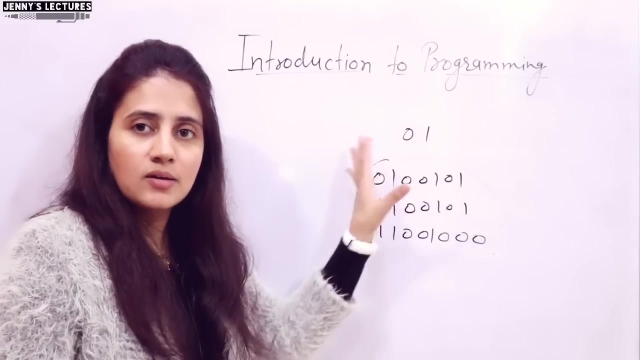 understand. Obviously computer will understand, because it is language of computer, right? So we write what Hash include stdioh, hash include conioh, then void main, then integer A, B, int A, B, then printf, scanf and everything, So that program first of all have to be converted. 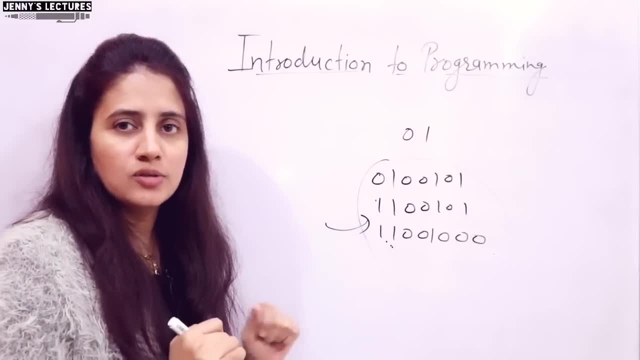 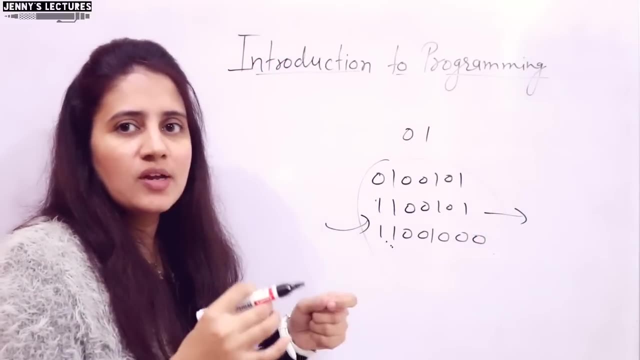 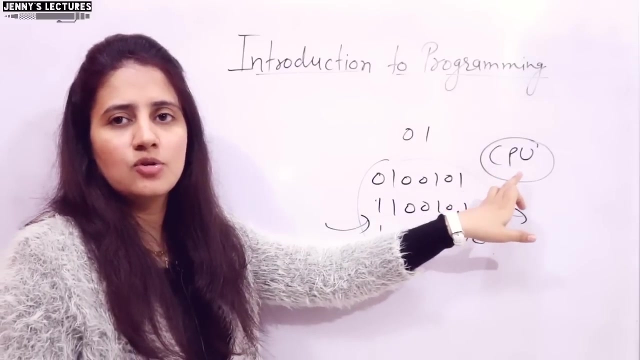 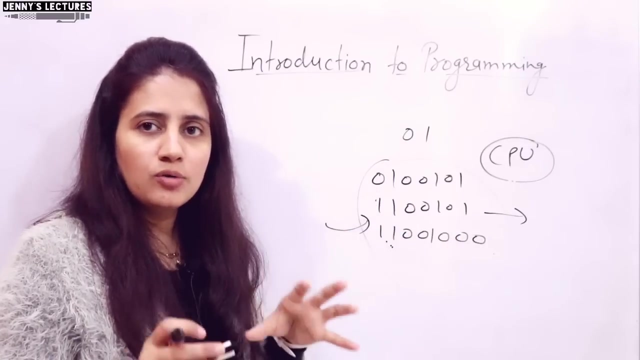 into this language, machine language, One form, And then computer will execute your program or, more specifically, I would say CPU, because it is what? Processor, central processing unit, This is processor, This is, you can say, heart of computer: The calculation, the computation, the task which you need to perform on computer. 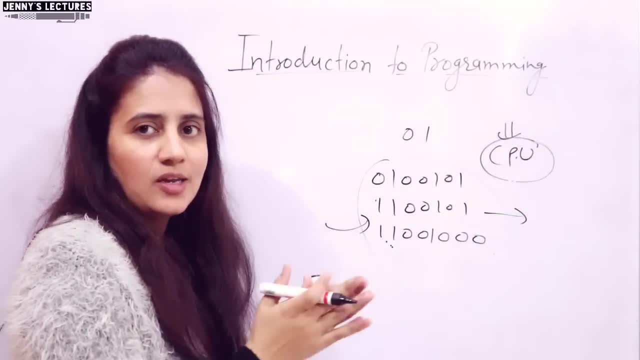 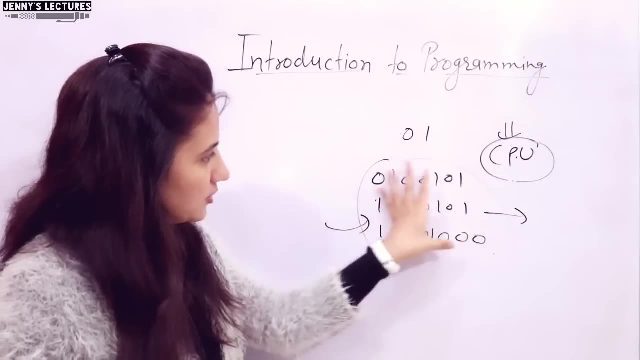 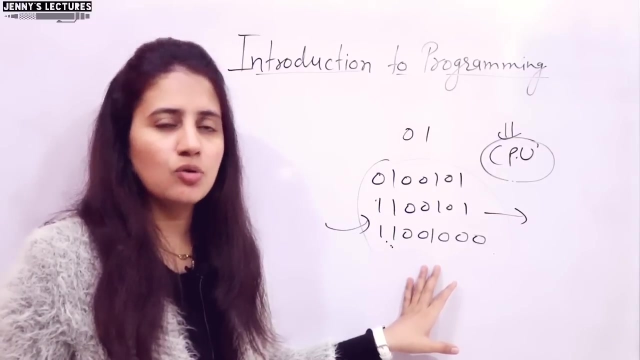 that is going to be performed by CPU. More specifically, if I will say: then CPU will give you output right. So if we write program in this format, this is what Machine level language- I hope you have heard about machine level languages, assembly level languages, then high level languages or low level languages. 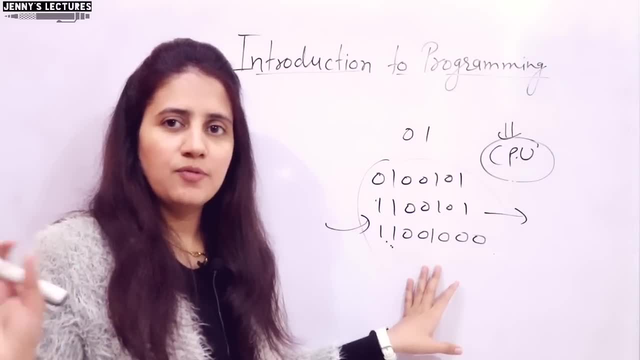 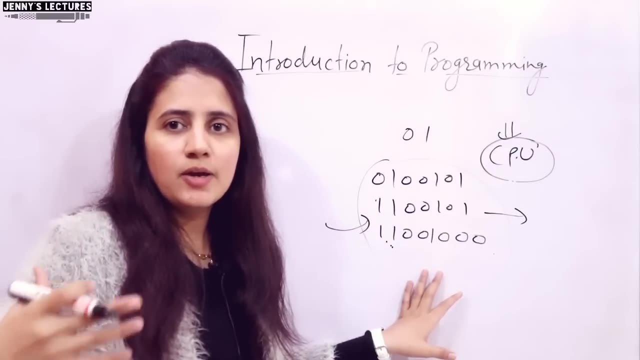 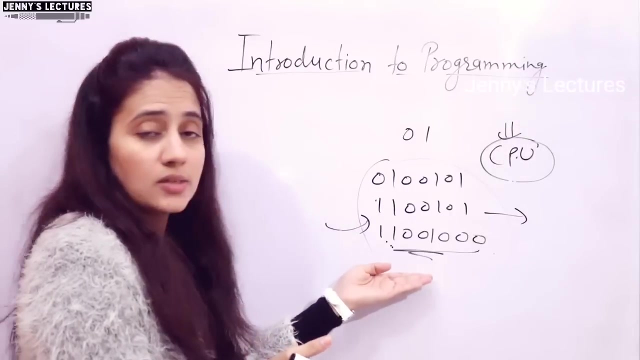 middle level languages right, But we will generally prefer to call high level languages right. High level languages means the C, C++, Java. These are understandable by human, because if we write this, if we see at this code, then we are not going, we will not understand what is this. This is machine level language. 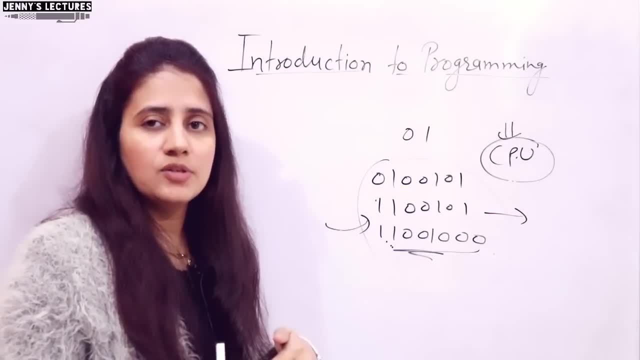 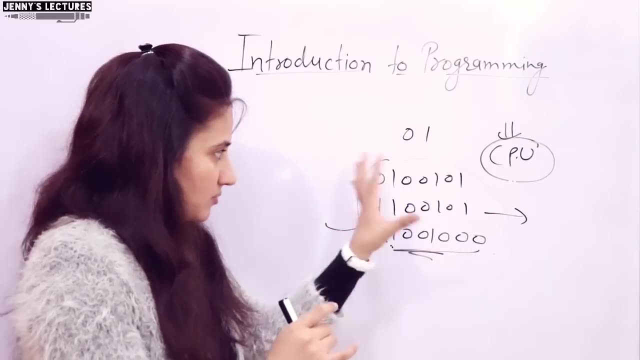 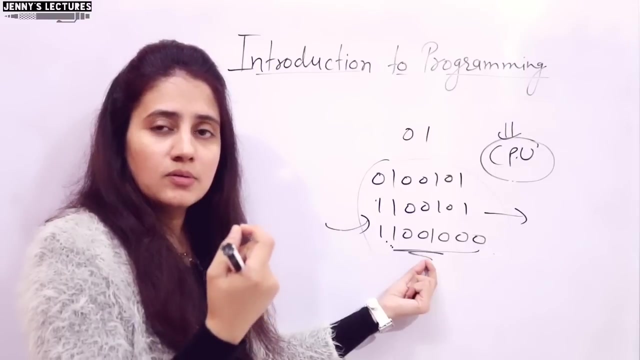 language, right, but before invention of these high level languages, they used to write programs in this format. see, you can imagine how tough it was at that time to write program in this language, machine language, because, see, and this is what this is according to you know, those cpu architecture. 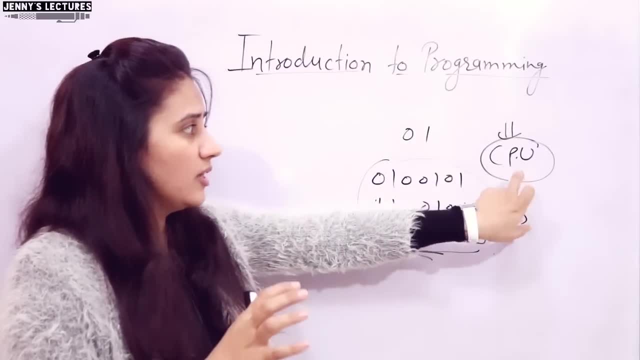 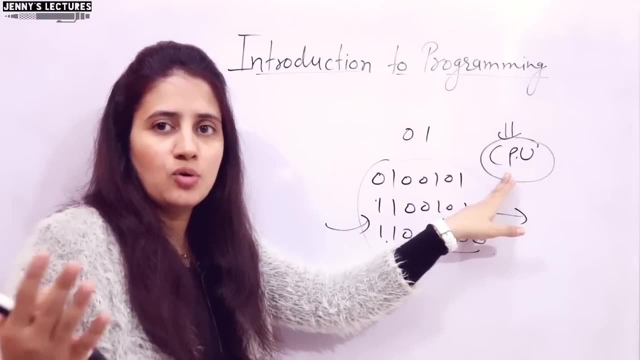 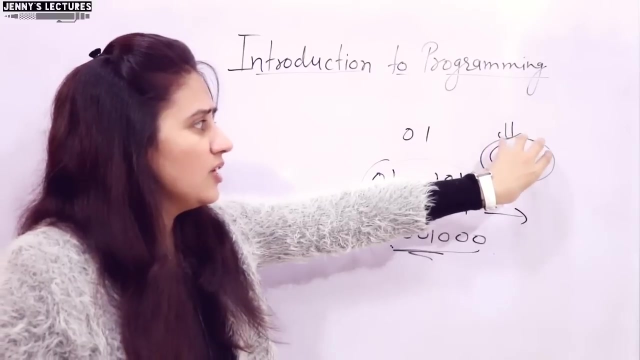 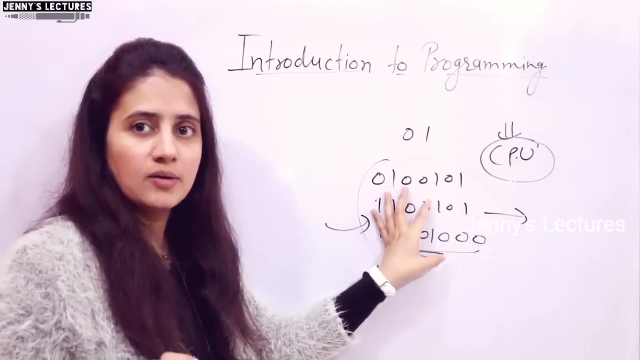 some set of specifications are there, which some architecture is there which cpu follows? i think you will, or maybe you have studied the subject coi, computer organization and architecture, in that you must have studied those architectures right. so according to those specification, those architecture of the cpu, this code will differ. it means it is machine dependent in one computer. 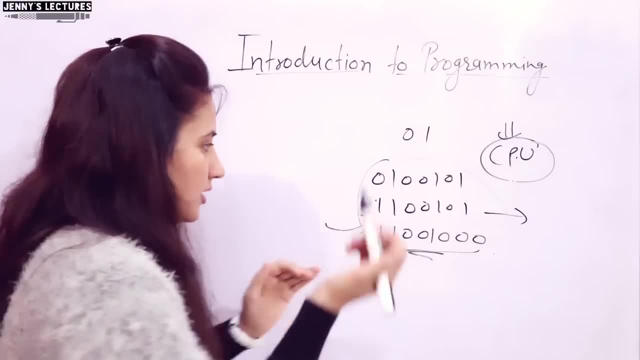 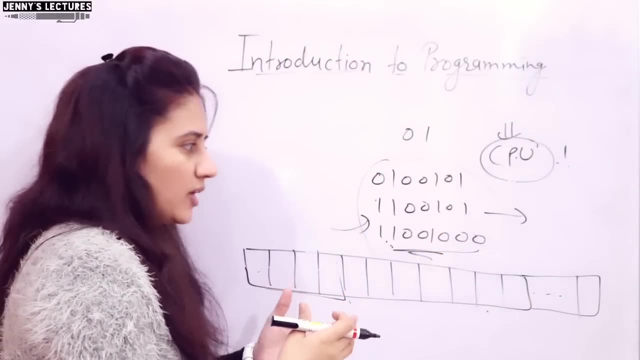 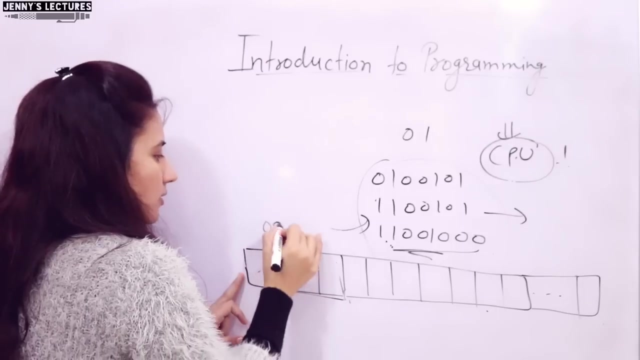 the same program, like addition of two numbers, let us suppose in at one cpu right. suppose according to this cpu architecture of the specifications the instruction can be given in twenty bits, like twenty bits right and first four bit are for operator. i hope everybody know like i suppose i am. 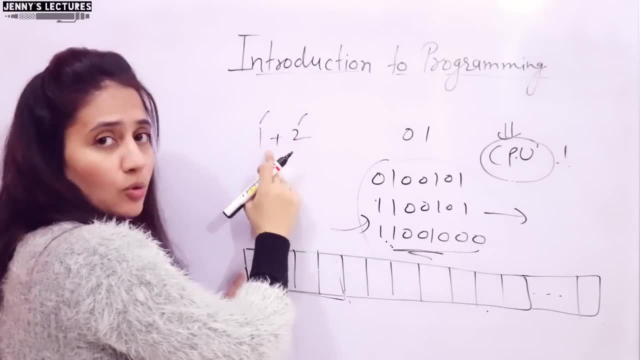 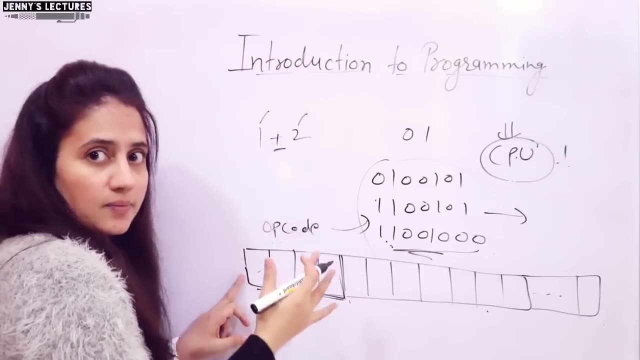 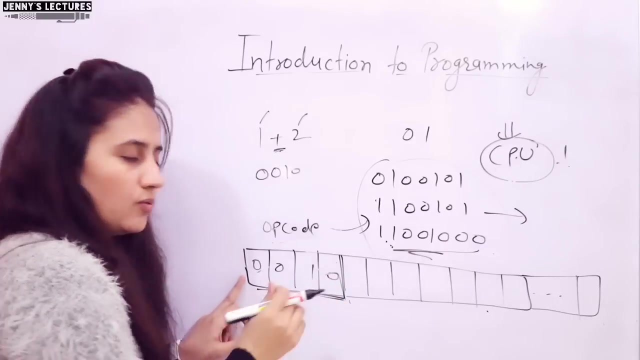 writing one plus two. one and two, these are operands and plus is operator. here we write as opcode. suppose these first four bits are for this plus, to indicate this plus, and suppose here plus. i will write like zero, zero, one zero, zero, zero, one zero. so computer will learn. 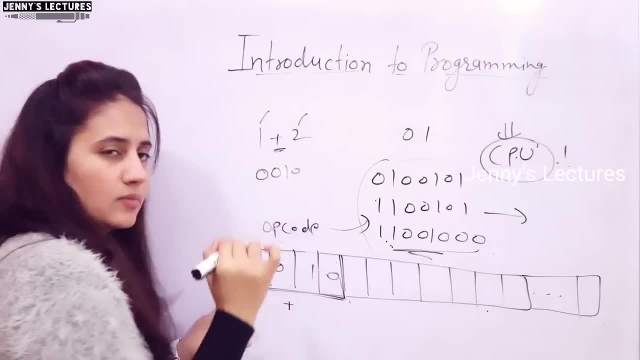 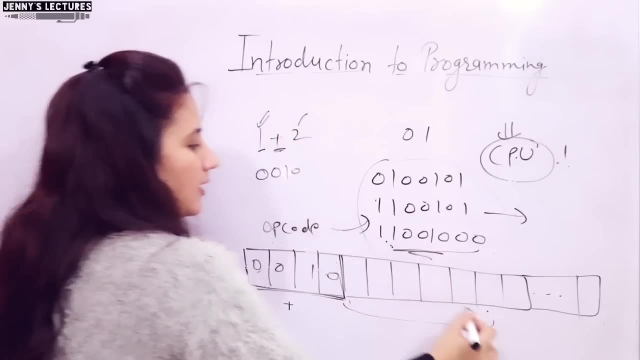 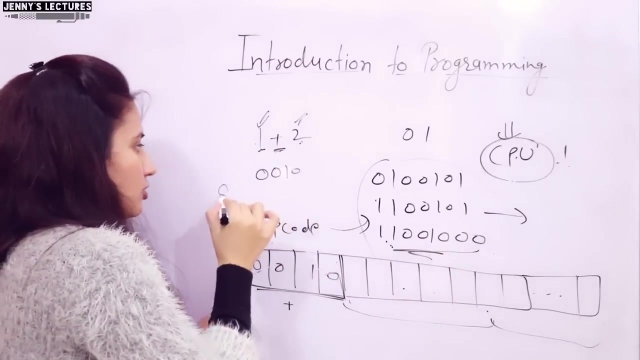 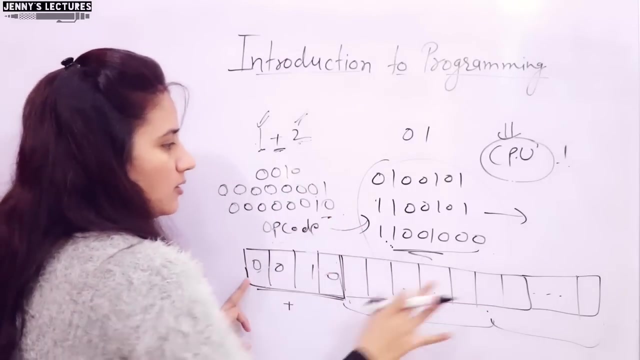 it will understand that this is for plus, that he has to perform plus operation, right, and then next eight bits are for one. this operand and next eight bit are for second operand. we will write these two operands into binary form, right, like zero, zero, zero, seven zeroes and one and two. how you will write this is two in binary form, so that we will write here: 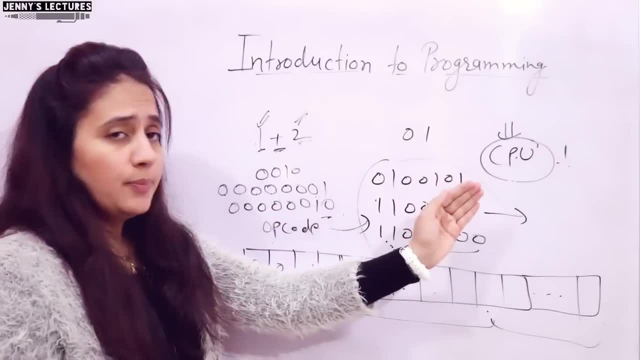 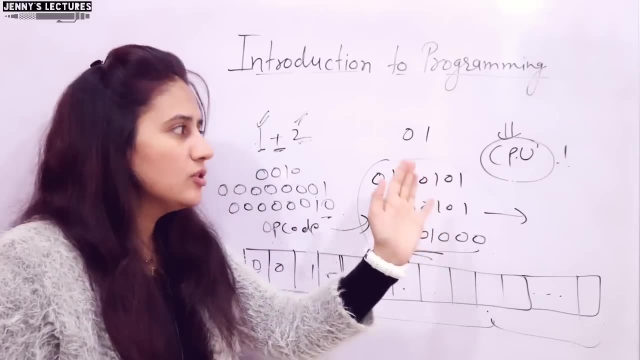 and when we submit this instruction, then the cpu will be issued. So i showed you it will present two in binary form inside the two, as the two in binary form perform addition of 1 and 2, and it will give you the result right And suppose the according to. 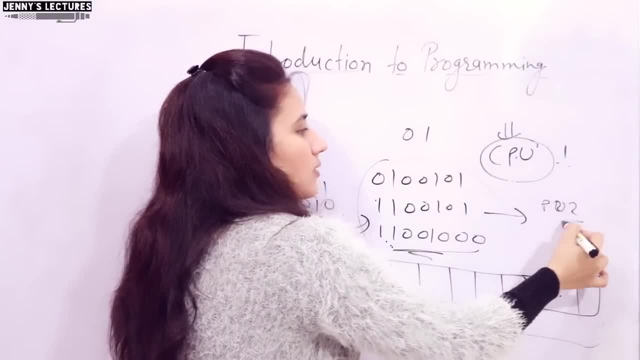 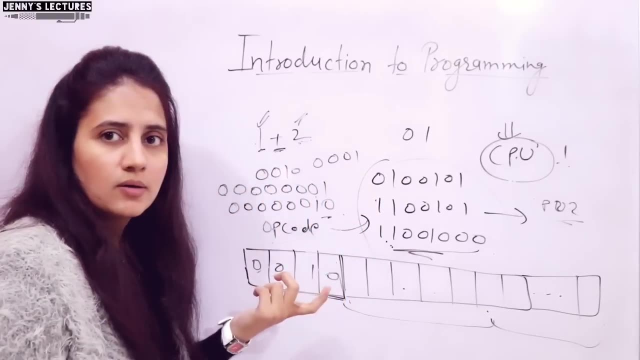 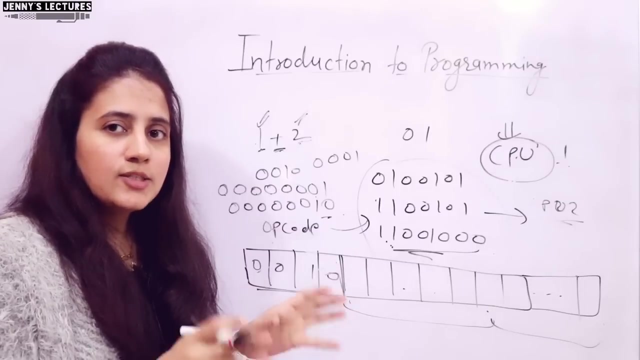 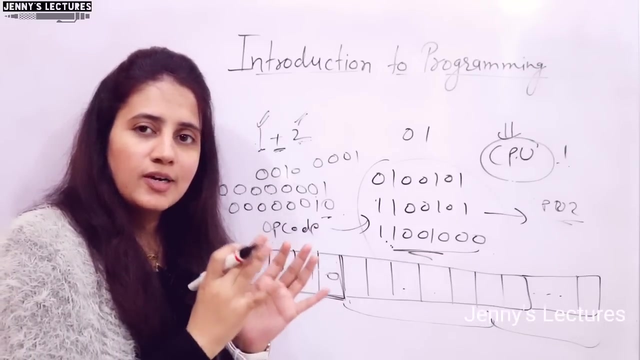 the specification of CPU 2. second processor may be there. plus is 0001 right or may be. the length of the instruction is something else, not 20 bits. So it is not easy to write programs in machine language because it is dependent on that machine to machine. So it is not, the programs are not. 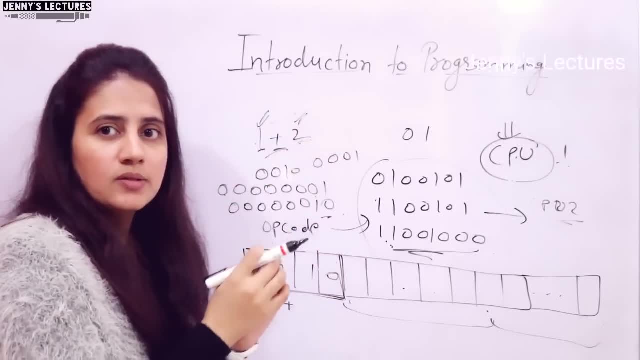 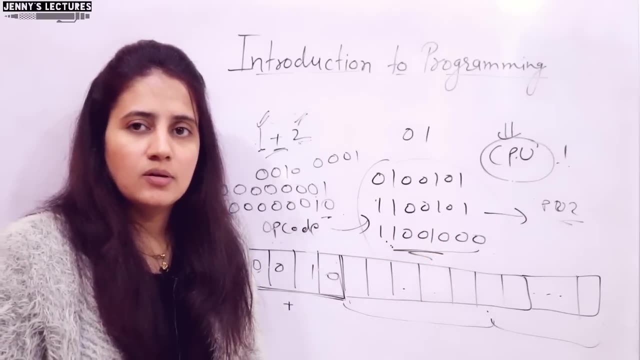 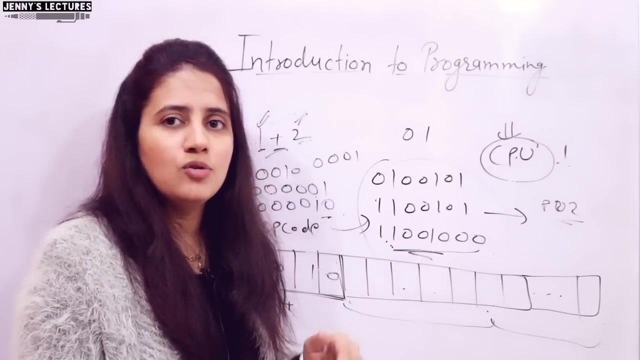 portable in one machine. if you are writing program for addition, then again you have to write, rewrite that program for second machine. it is not like that the same program will run on second machine. that is very difficult. then assembly level languages come. these levels we will discuss in a separate video with more details- and after that high level languages come to overcome these. 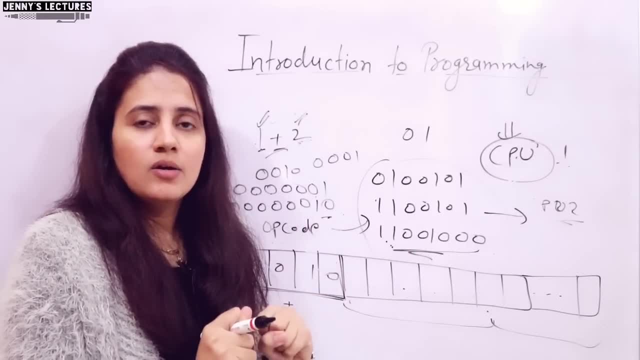 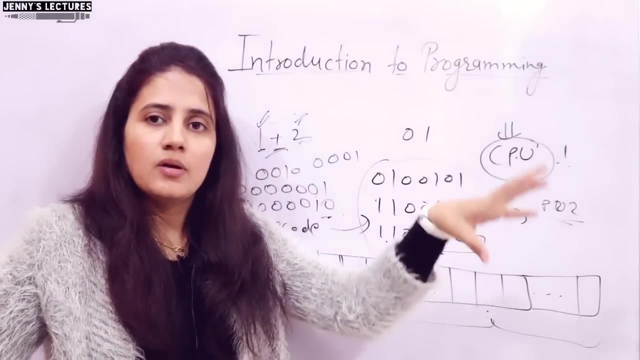 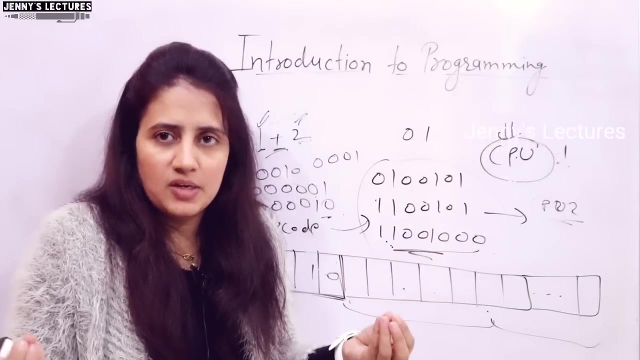 limitations, to add portability concepts, So that one program on one machine we write and that program can easily be ported to second machine, means we can. we can run that program, same program, on second machine also without any modification, or maybe you can say: with few modifications, right? So now let us discuss what. 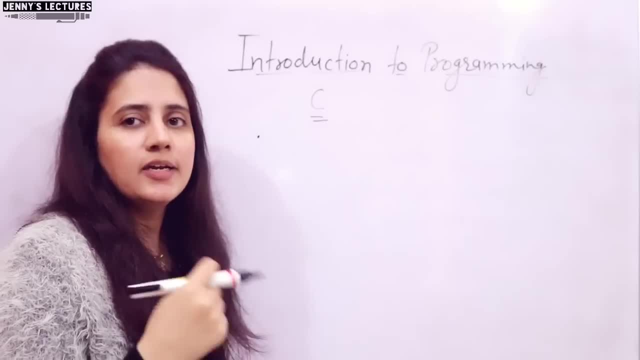 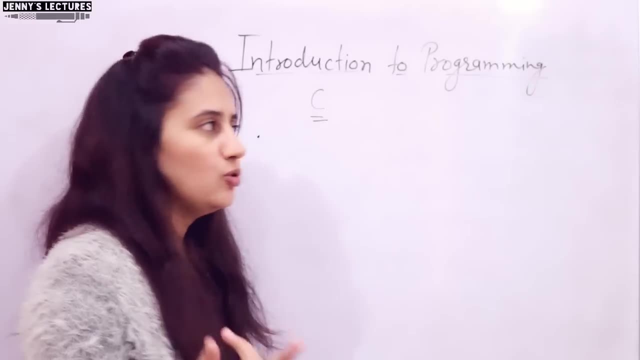 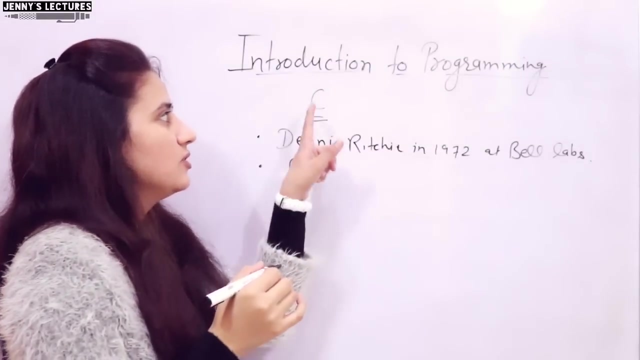 is C language. see, it was developed by Dennis Ritchie in 1972 where Bell laboratories, the headquarter of these Bell labs- are where in New Jersey, US, right, and it is before C the language was developed B language. so you can say C is what successor of B. 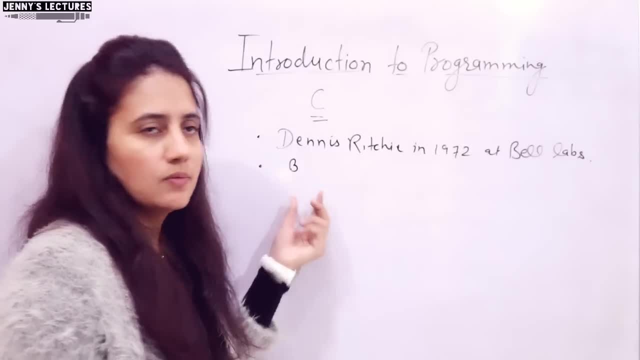 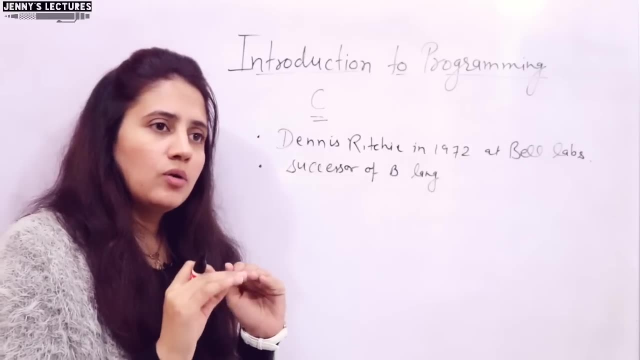 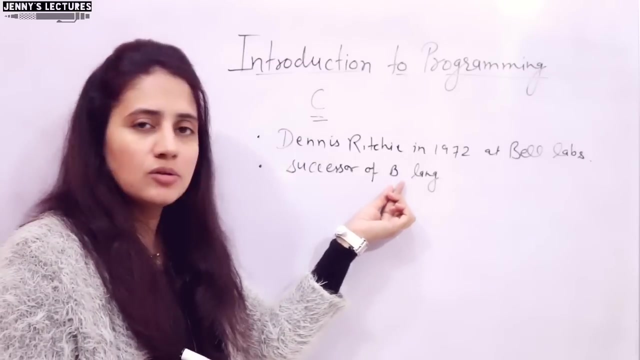 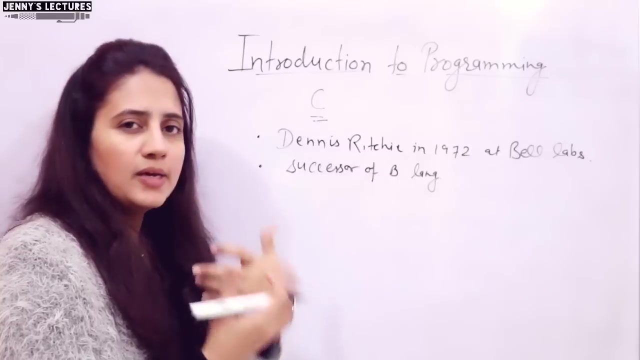 language. it was developed by Ken Thompson, right? Why C language was developed at that time? basically, the main purpose was to, you know, write operating system, that is, Unix operating system. that was already written in B language but there was some limitation. so, to overcome those limitations, because C was more powerful than B language, right? So they used to write the kernel of. 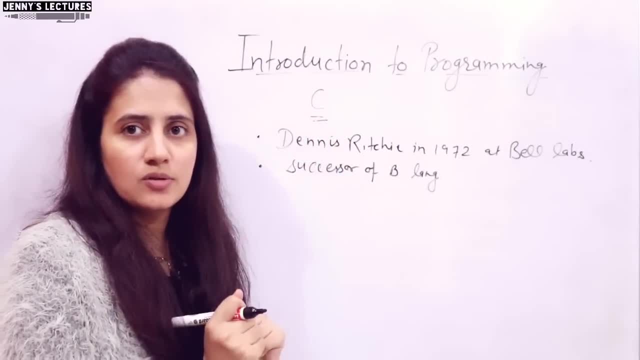 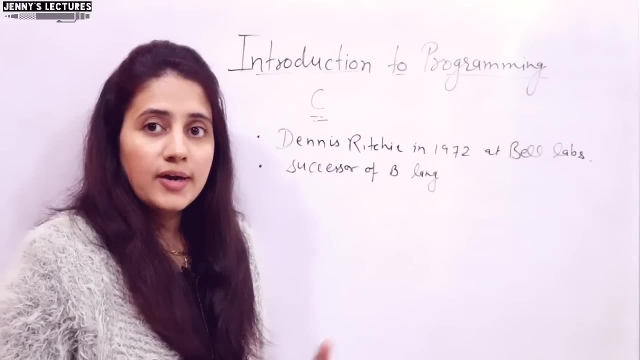 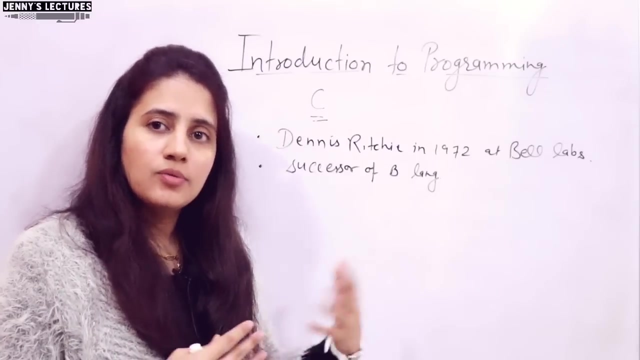 Unix operating system. they used this language C language. so C is basically you can say it's a system programming languages language. many softwares have been written in C language: oracle, Android- the core libraries of Android was written in C language. major part of web browser is written in C language, device drivers written in C language and then the kernel of the core libraries. 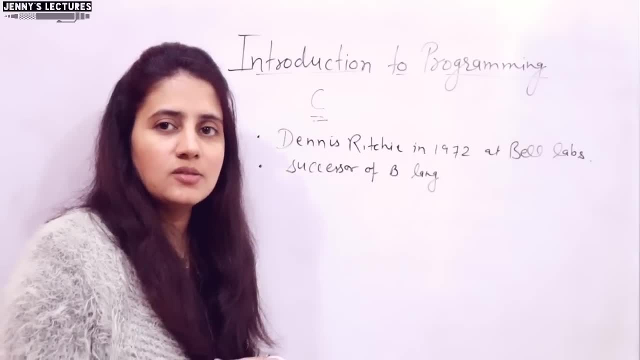 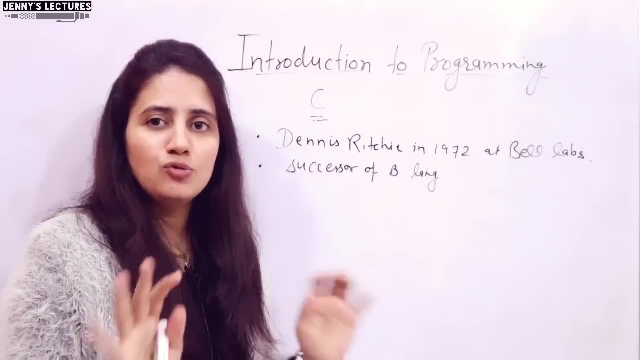 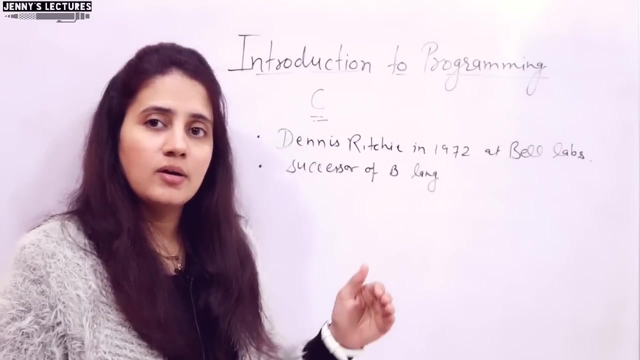 C language and Unix operating system. so C is, you can say, the most popular programming language, and during 1980s C was the most widely used programming language and in 1989 it was standardized by ANSI. that is why after that it is called ANSI C and see how the computer is going to understand what.